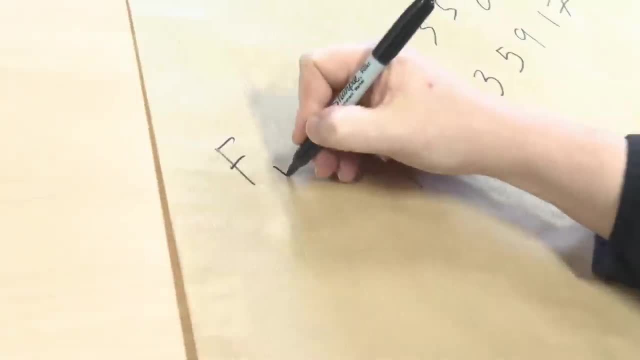 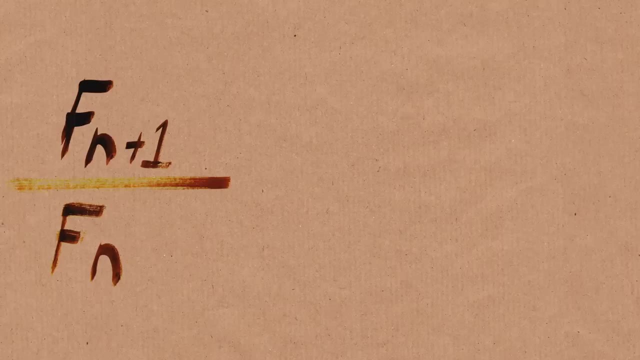 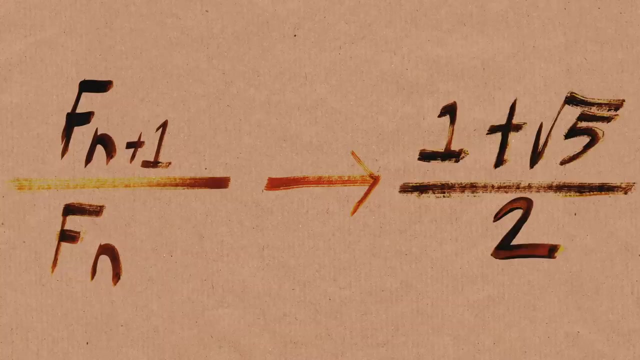 So it's called the Tribonacci numbers, Let's call this fn, and so this is the Tribonacci tn, And you have that. fn plus one divided by fn goes to the golden ratio. So we can also do the same thing with the Tribonacci numbers. 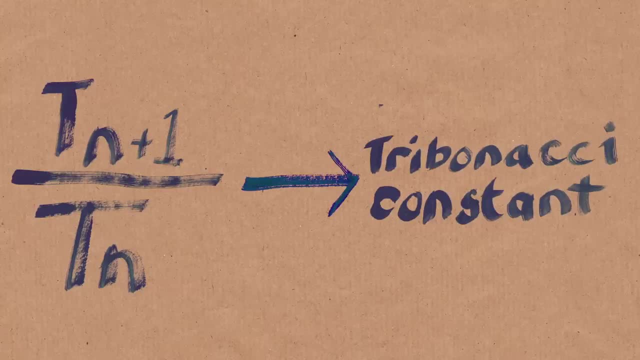 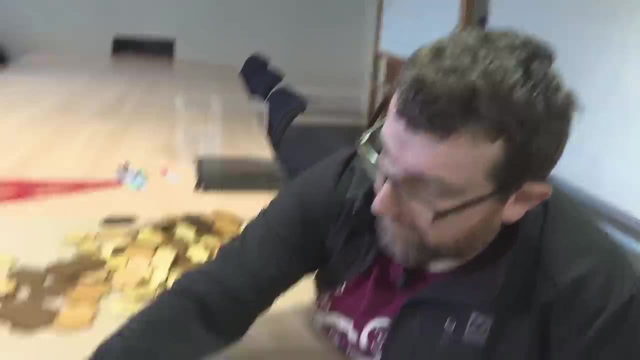 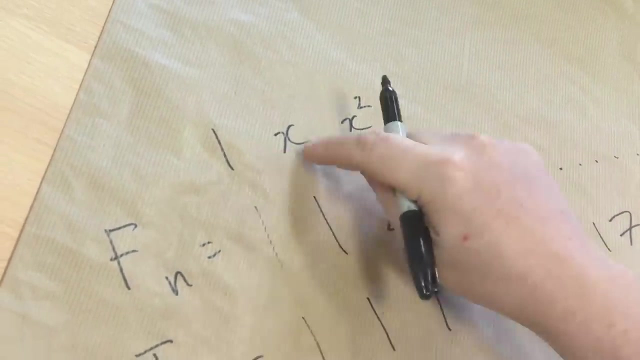 but they go to what's called the Tribonacci constant With the Fibonacci numbers. one of the ways we can sort of think about how they're going to end up is say: well, let's start this one: x, x squared, and x squared was equal to the two previous ones together. So here, 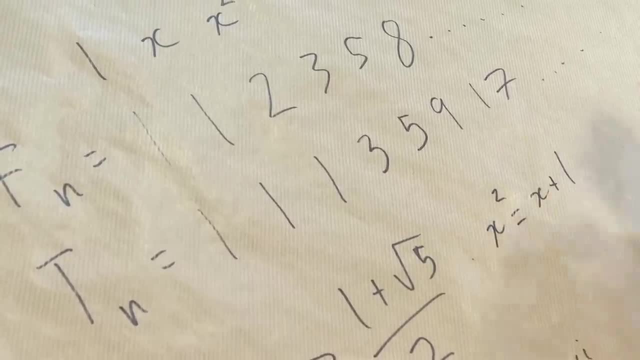 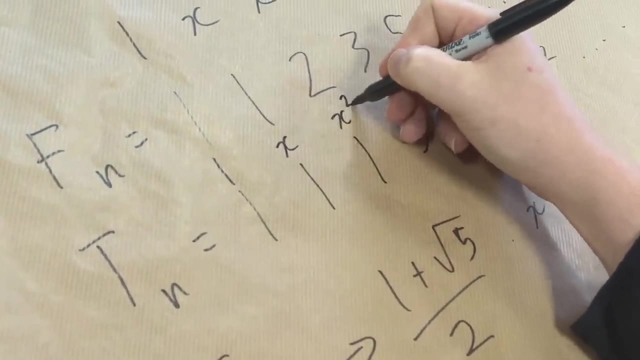 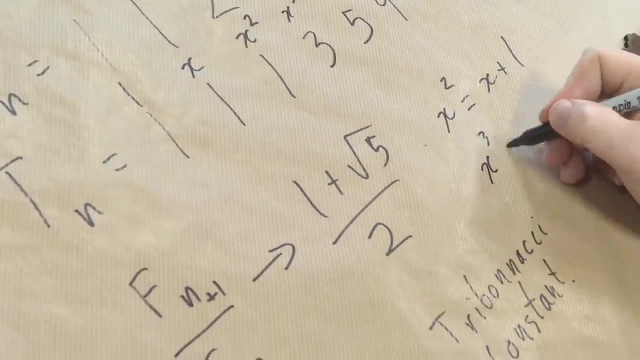 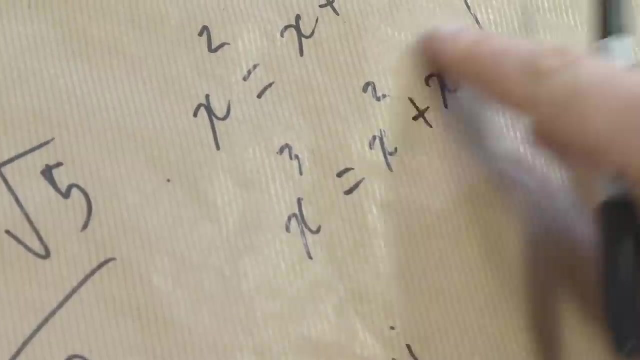 is: x squared is equal to x plus one. Here we're adding the three previous terms, So we get 1 x x squared. This term is going to be the sum of all three, So it's x cubed, and now we have x cubed is equal to x squared plus x plus one, And so that's a polynomial. 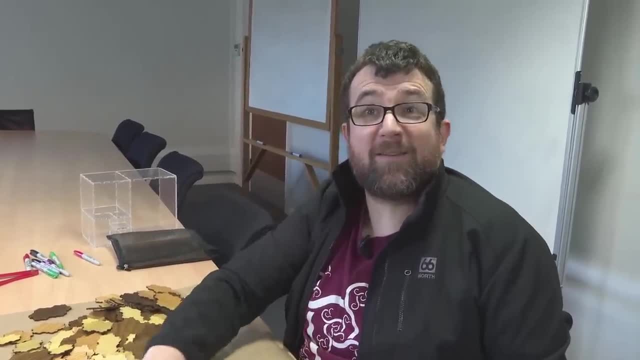 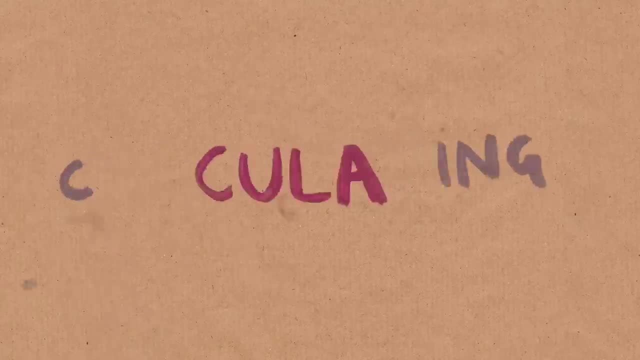 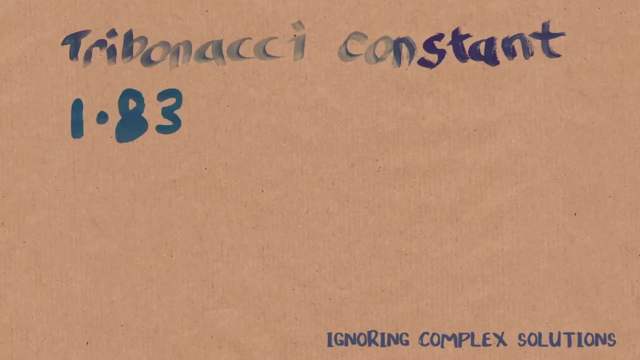 Whilst I can reasonably well solve quadratics, Rubik's have a far more messy to solve, so I want to get a calculator to do that. So this gives us 1.83929, and that's gonna Tribonacci constant, Tribonacci constant. 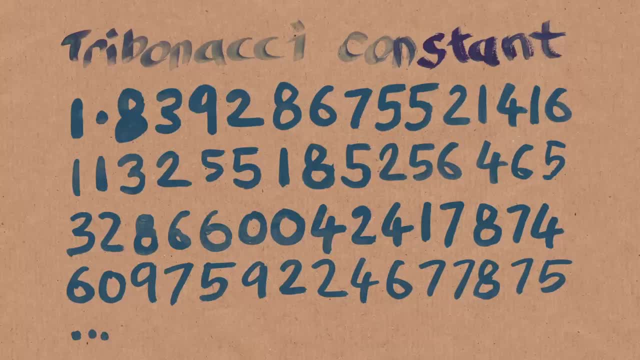 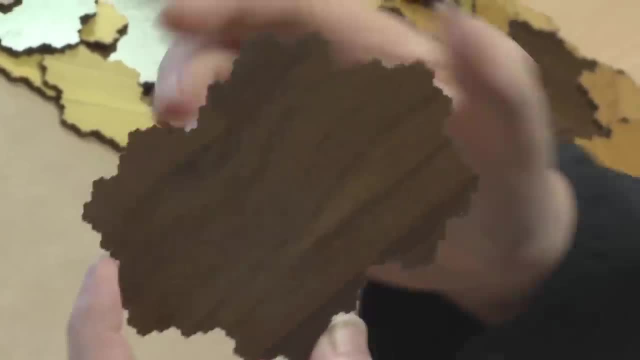 I'm assuming there's a 4-Bonacci constant and a 5-Bonacci- They're called the n-Bonacci's, And so here I've got an interesting shape. It's got a fractal boundary going around it. Well, it's got a nice property to it. 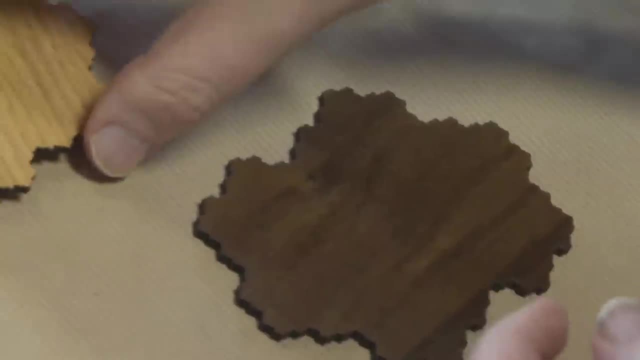 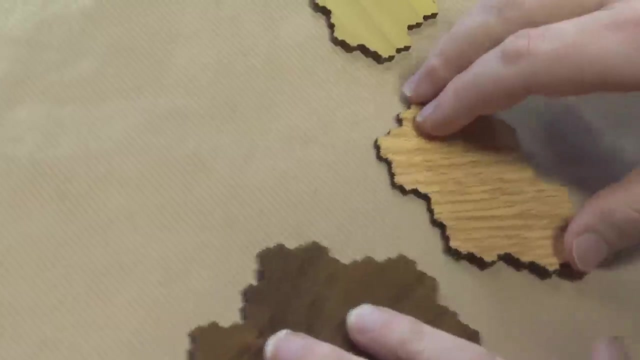 So I've got this tile here and this is the same shape but a little bit smaller. And then I've got again the same shape, but smaller- The edges of these, if I can find it. I have to get them the right way up, and there we go. 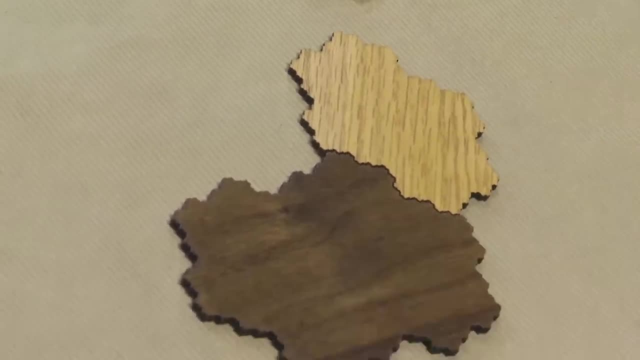 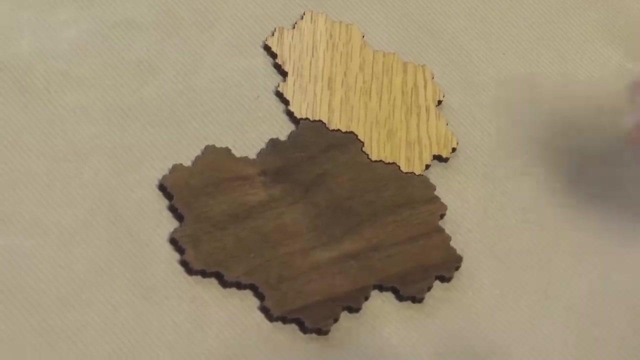 So the edges are such, so this shape at different sizes actually fits onto itself, And that means that these edges might must either be straight lines, which they're clearly not, or fractal. It's not a fractal itself, But the boundary is a fractal. 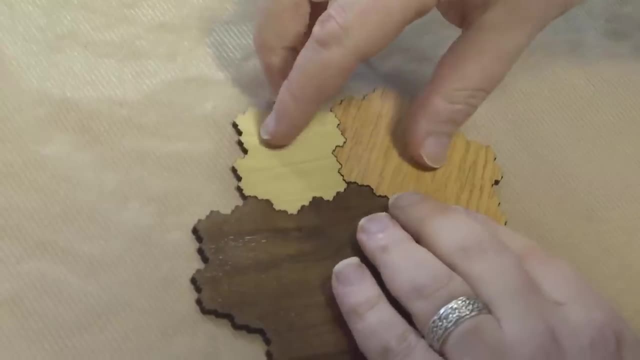 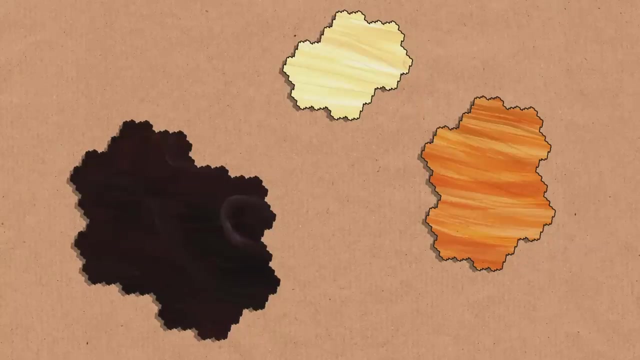 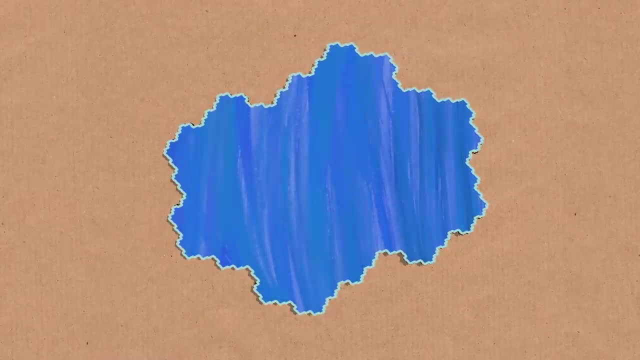 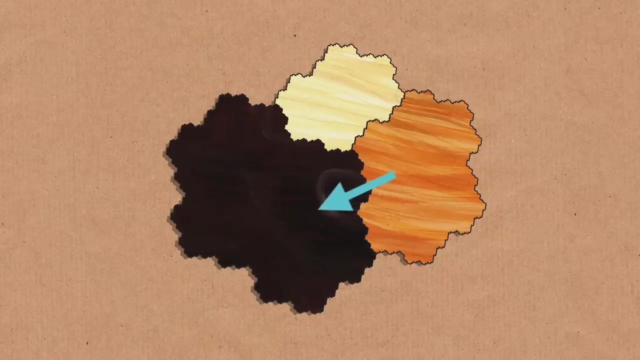 So now I will take a third shape and put them there and magically I have my same shape. These are three sizes of this one shape, and when I put those three together I get the same shape. If this one scales up to this one, this one scales up to this one. 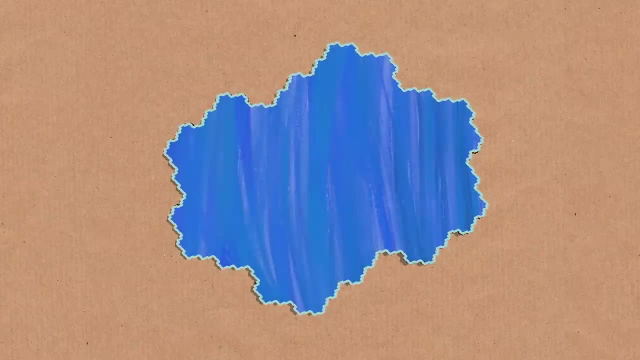 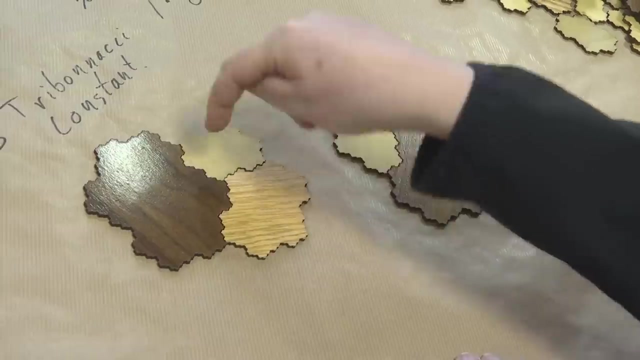 and then this one scales up to this one, and then this one scales up to the whole thing. I can take this one step further. So what I've done here is make a larger version of this object. So this piece here becomes this tile here. 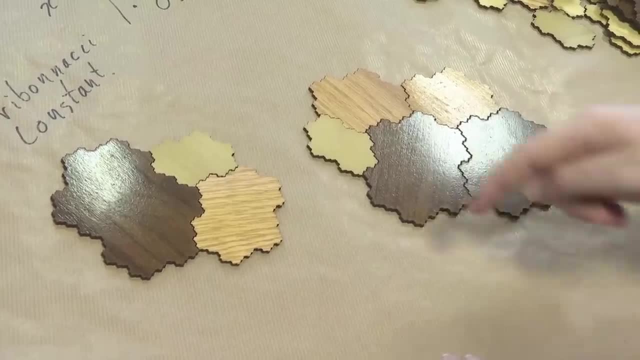 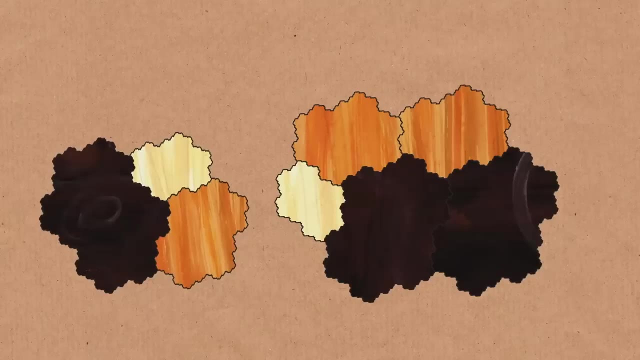 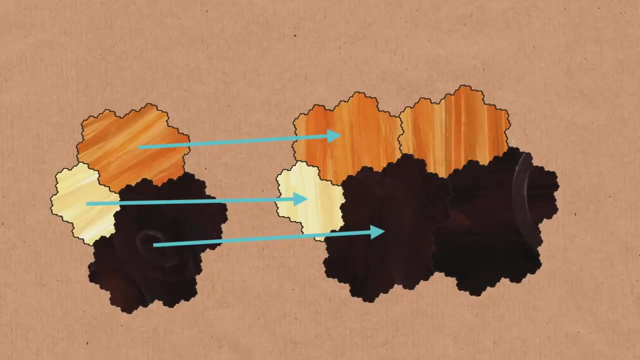 This piece here becomes this tile here, And then this tile here is replaced by the whole piece here. It's the three tiles. If I rotate this to there, you see that this is just these three tiles. So now we can imagine doing this another time and another time. 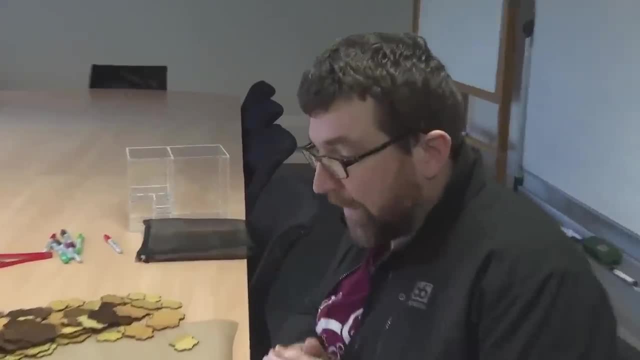 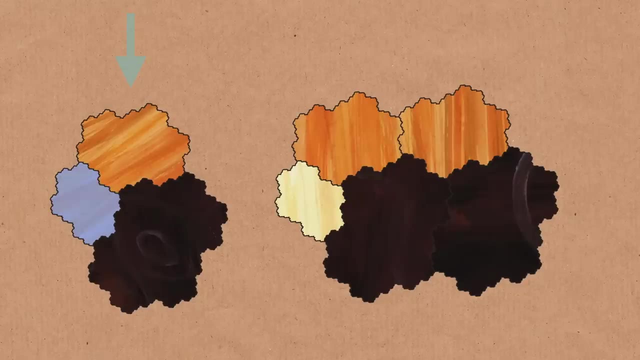 We can get larger and larger regions, We could ask: well, how many tiles am I going to have in them? Well, this pattern is made up of one of the smallest tiles, one of the medium tiles and one of the large tiles. 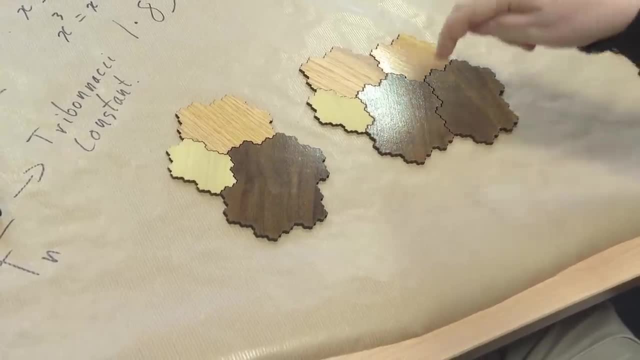 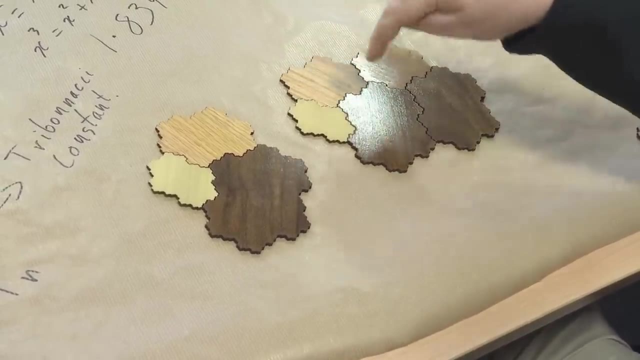 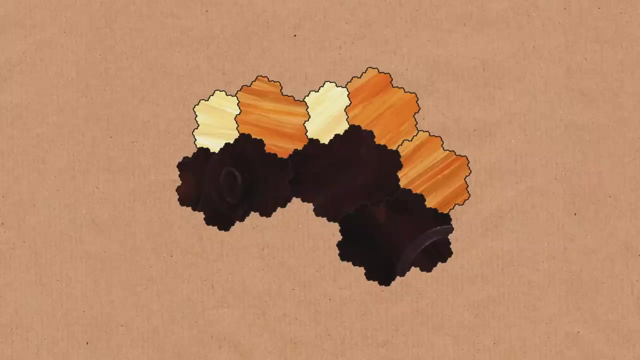 This is made up of one medium, one large, and then one of the scale size beyond large, which itself is made up of one small, one medium and one large, And when I go to the next step up, I'm going to have one copy of this, one copy of this and then one additional large one. 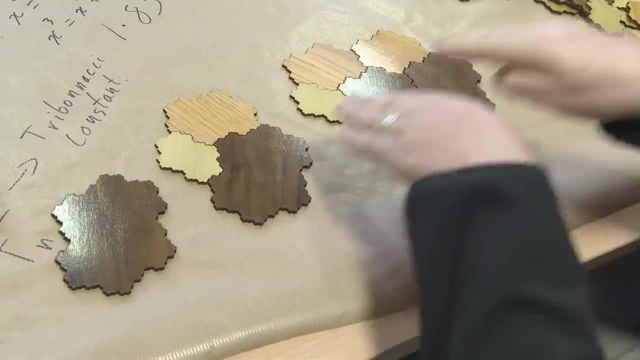 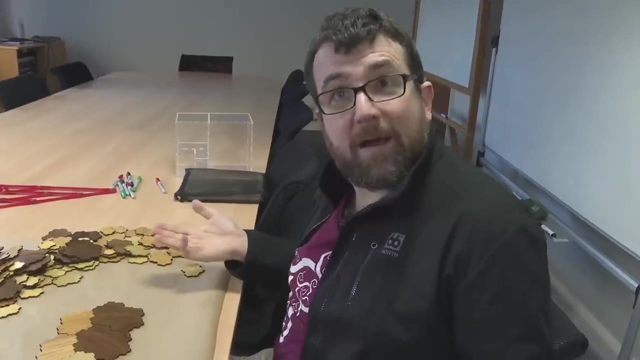 So, at each stage, I'm going to take the three previous pieces, put them together to get the next one up, And so what are we going to have? Well, it's back over. here. I have my one, one, one. 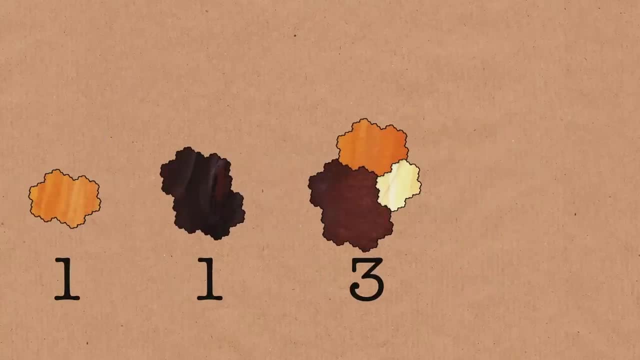 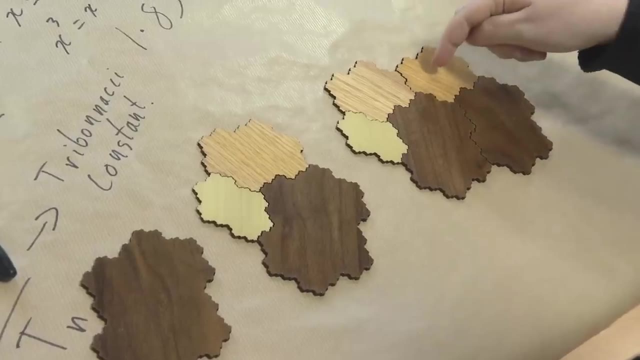 I put those together, so I get three, One, One and three give me my five. The next one up is going to be my five, my three and my one which is going to give me nine, and so on, like that. 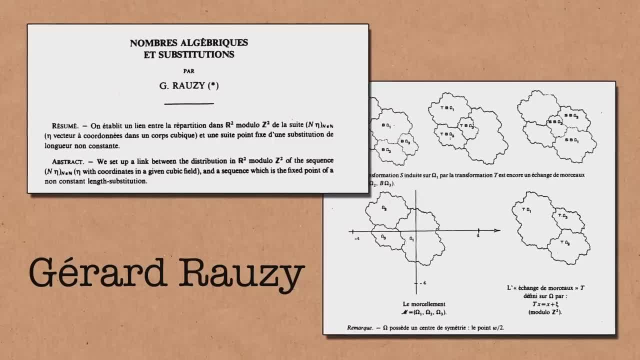 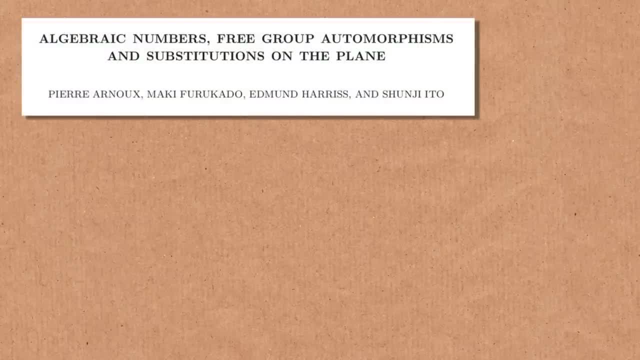 So this shape is called the Rousey fractal and it was found by Gerald Rousey. The interest is sort of studying how matrices act on three-dimensional space And there's a lot of nice theory for how, for certain properties of how, matrices act. 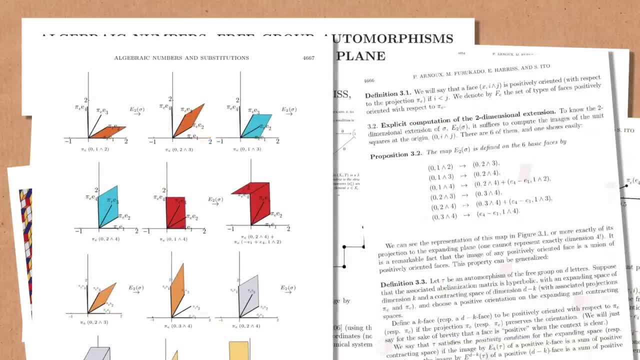 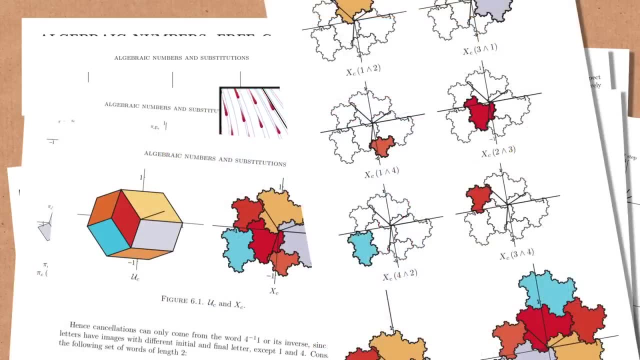 on two-dimensional space, especially a matrix which has one expansion and one contraction. What that will do is you have these things called eigenvectors and you pull down in one direction and you expand so that everything gets squashed down and pulled out. 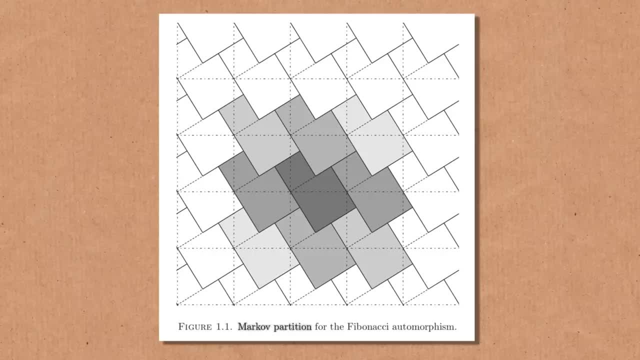 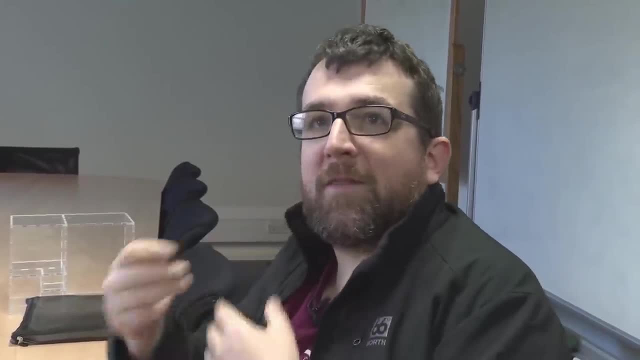 There's a whole theory in that, called Markov partitions, which basically have nice properties. As you get pulled down and smeared out, you can turn that into a nice periodic property. People ask: well, what about for the cubic case, when we're dealing with three-dimensional space? 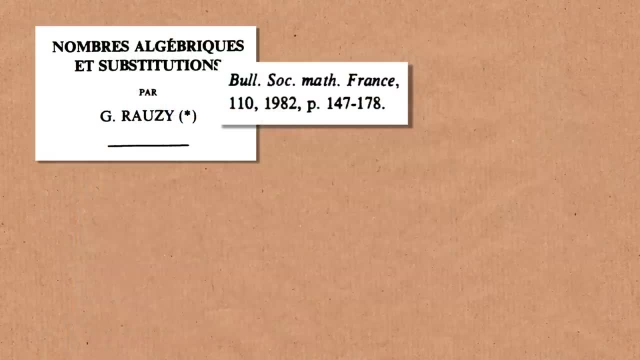 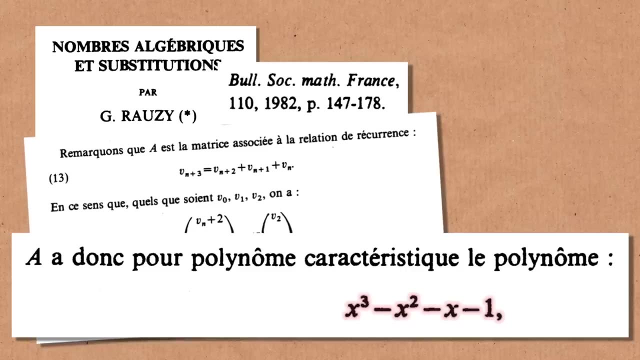 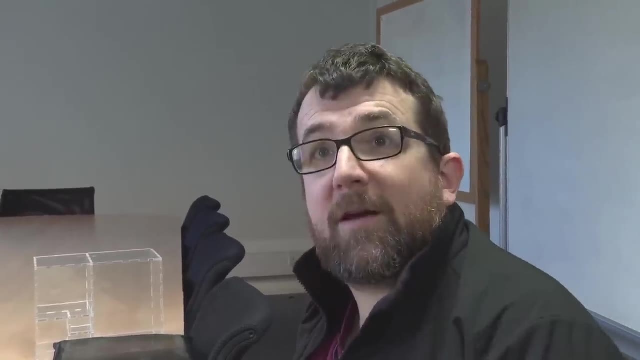 So the specific matrix you're studying here has as one of its eigenvalues this number, the Tribonacci constant. And so, because the Tribonacci constant is turning up in the thing you're trying to study, that's how it turns out in these tiles. 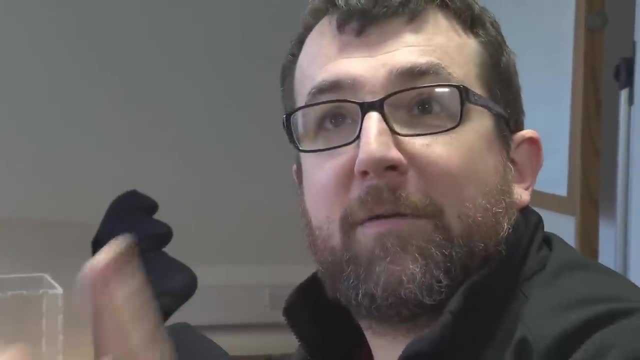 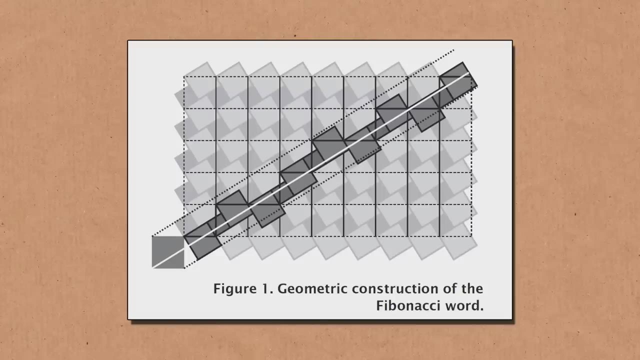 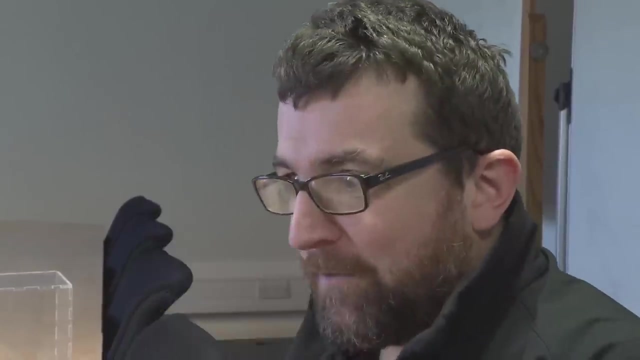 And the golden ratio and the Tribonacci numbers are really important in the study of the two-dimensional space And so when you go up to three dimensions you have to deal with cubic things. It's quite natural. It's sort of almost the ancient Greeks who felt that a cubic number really was a cube. 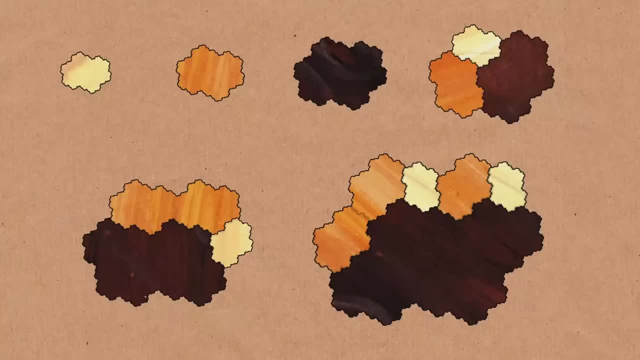 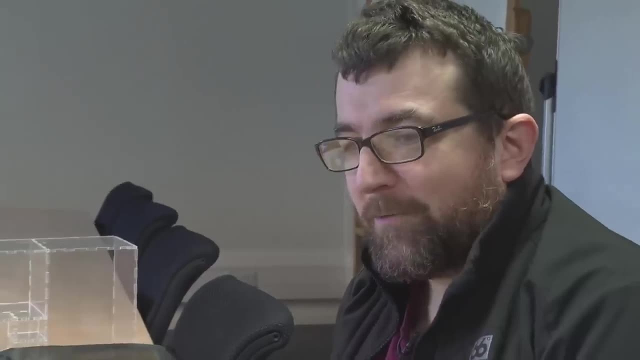 So they didn't. some people say they didn't even believe in four powers. When you're dealing with three dimensions, you naturally have cubic stuff. Do they exist in sunflowers and things like that? They don't exist in nature in the way that they just like. the Fibonacci isn't quite as popular in nature as it's meant to be. 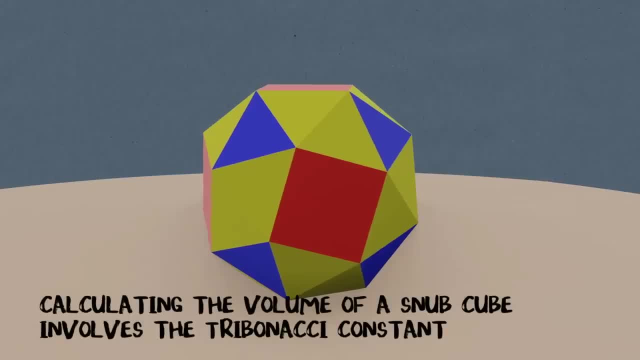 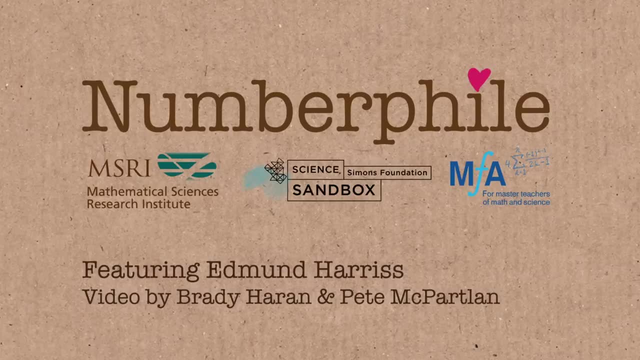 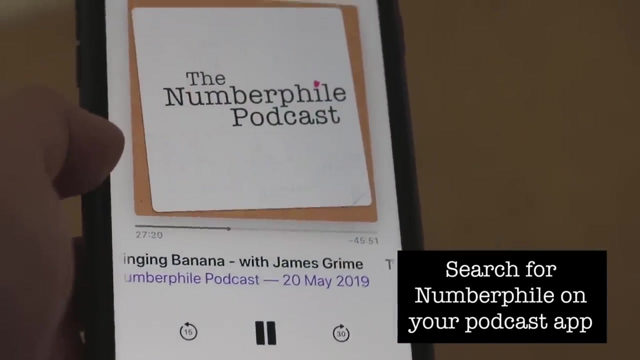 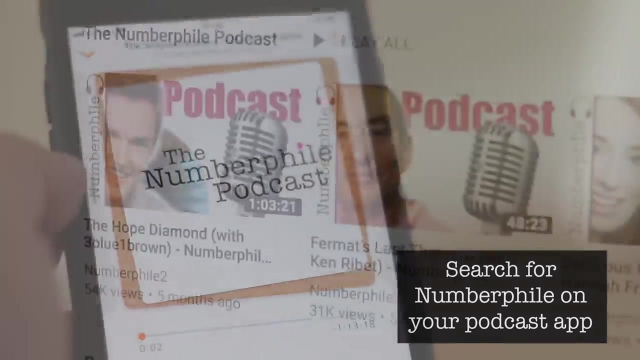 The only place beyond this that I know of them is an object called the snub cube, which is quite an attractive little polyhedron. I'll leave a link to it in the description.